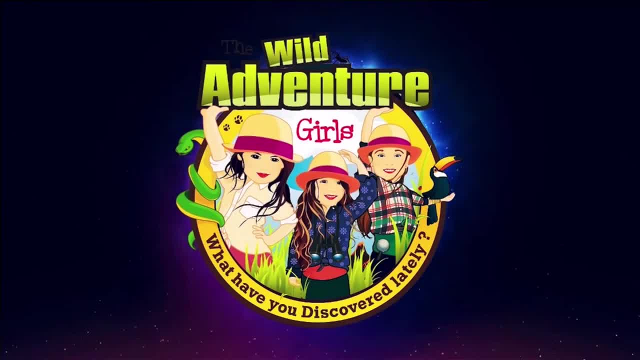 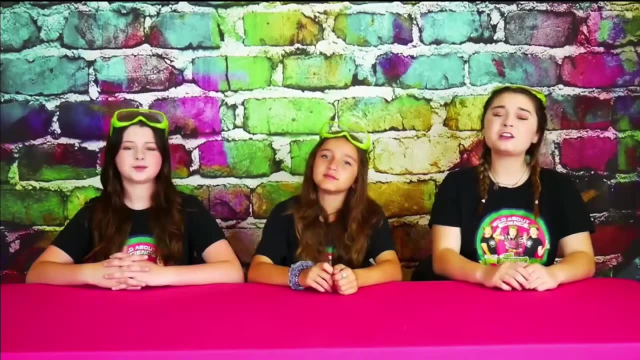 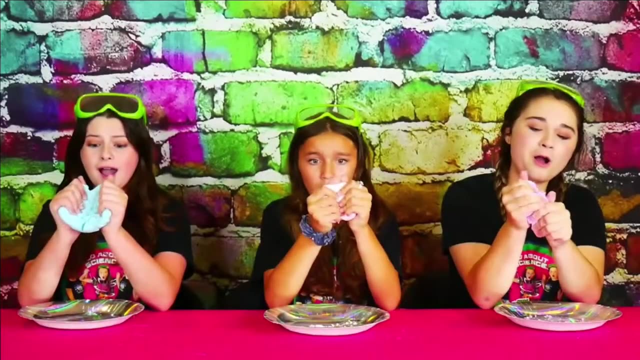 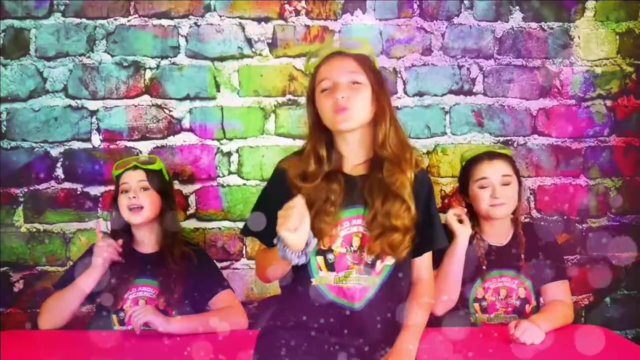 Hi, we're the Water Beach Girls, And we're the Water Beach Girls. It's our channel. Today we're going to show you how to make a super fun and really magical unicorn cloud dough. Oh yeah, baby, Whoa, This is so soft. From the inside it looks like a cloud, But first we're going to need a few unicorn things. 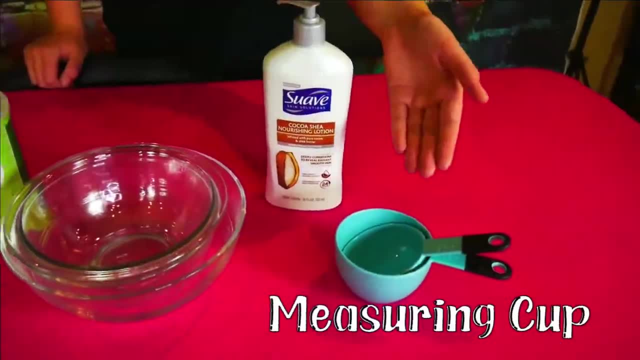 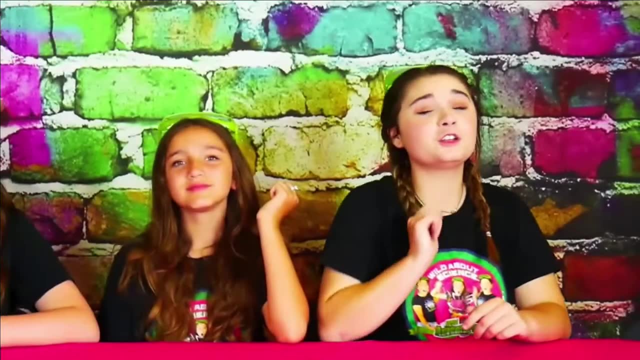 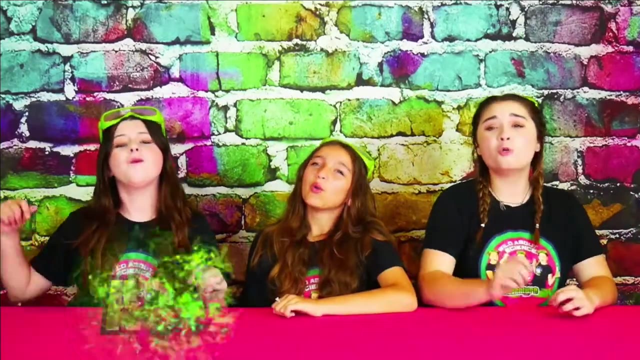 We will be using lotion measuring cups, glass bowls, cornstarch, unicorn glitter and unicorn food coloring. If you're new to our channel, I'm Angelina, I'm Scarlet And I'm Annabella, And together we're the Water Beach Girls. 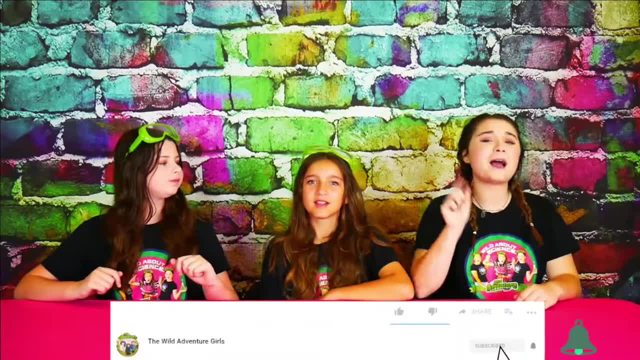 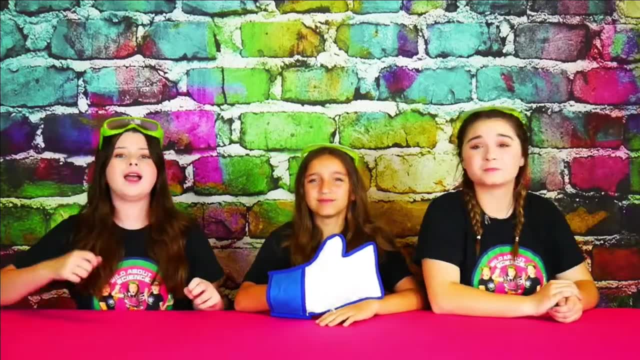 Subscribe to our videos. We'd love for you to pound subscribe button, Ring that bell And smash that like button And under five seconds. Do you think they can do it? Heck yeah, Ready. Five, four, three, two, one. 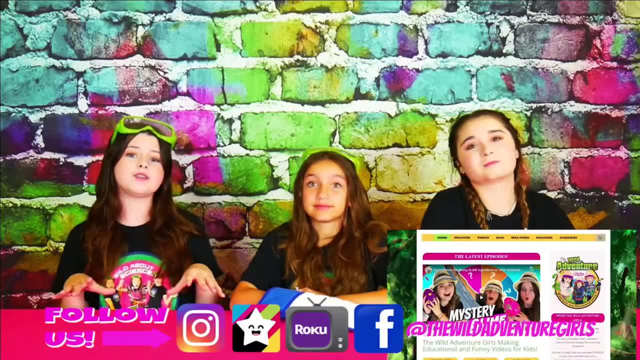 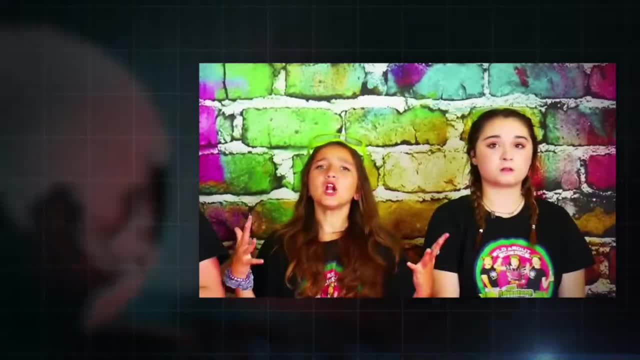 Great job, guys. If you haven't already, make sure you head to our website at thewaterbeachgirlscom And come on any one of our blog posts Hashtag Water Beach Squad, letting us know that you did it. We interrupt this video for an important announcement. 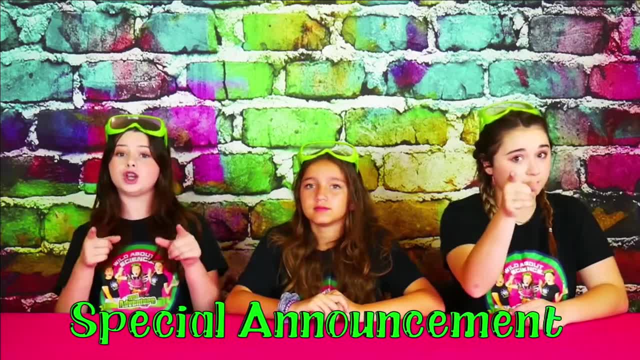 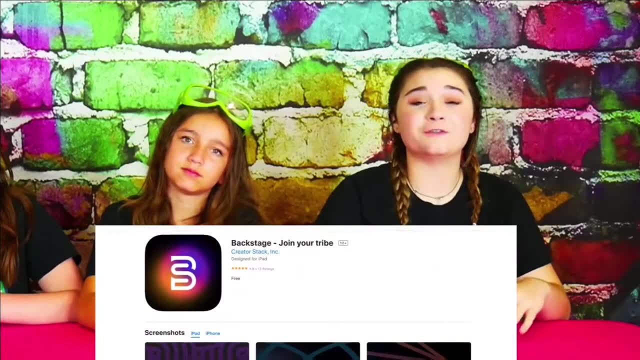 Coming soon. look for a special announcement where we invite you, our Water Beach Girl Squad, to our backstage. What is backstage Backstage is exclusive for our fans only And you can see all that fun, All the fascinating behind the scenes stuff. 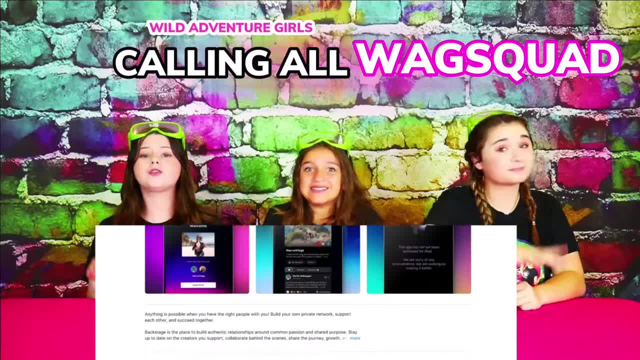 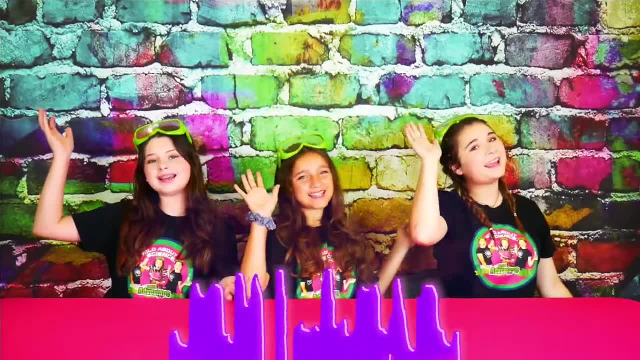 And you get to participate in challenges that aren't found anywhere else but backstage. Okay, back to our video. Okay, let's get ready Now. first thing we're going to do is take half a cup of lotion and pour it to three separate bowls. 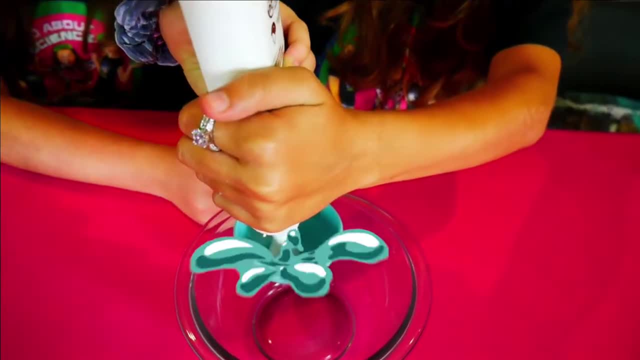 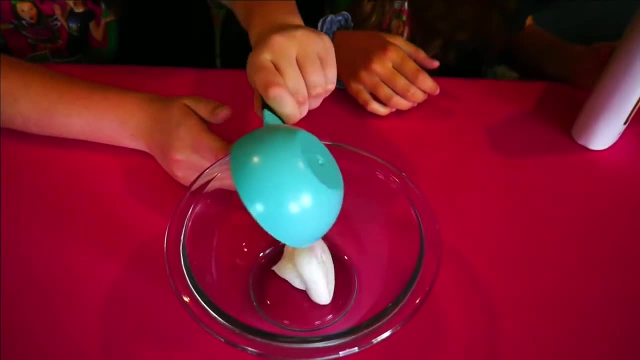 Here comes our half a cup. This smells a lot better than glue. It does, Eww. Oh, it smells so good It does. We're going to dump it in our bowl- Eww. Next, we're going to add some pretty unicorn food coloring. 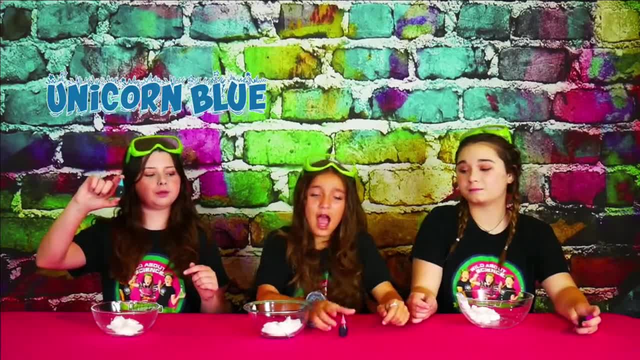 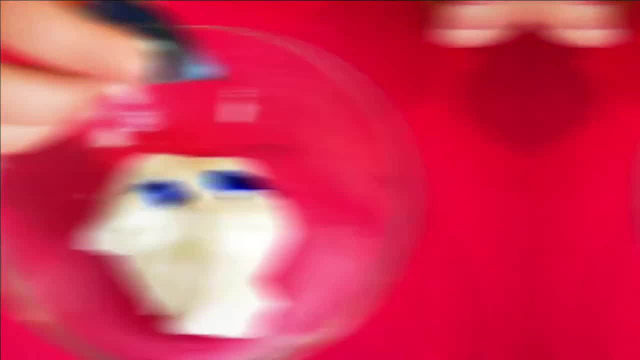 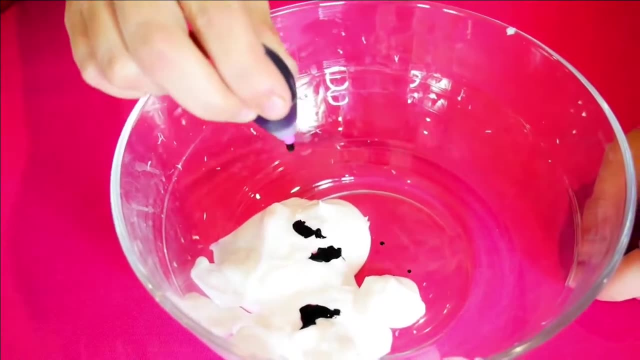 I'm adding a pretty unicorn blue, I'm adding a pretty unicorn pink And I'm adding a pretty unicorn purple. That's my unicorn blue. That's my pretty unicorn pink. Now for my unicorn purple. This is going to look so cute. 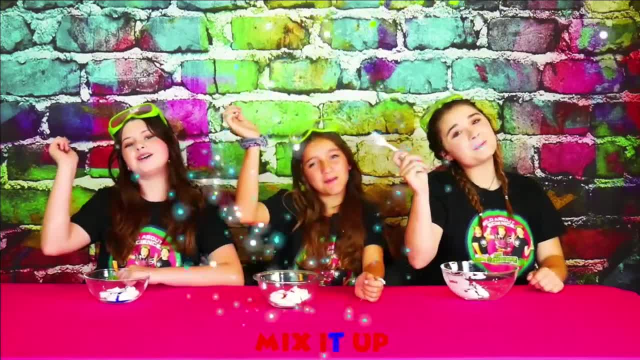 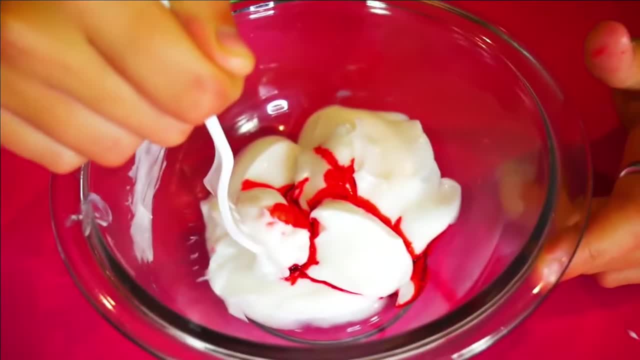 So cute. Now it's time to mix it up. Let me mix my unicorn blue. Oh, that is so pretty. Oh, Here comes my pretty unicorn pink. Oh, that's so nice. Oh, it's going to be such a good pink. 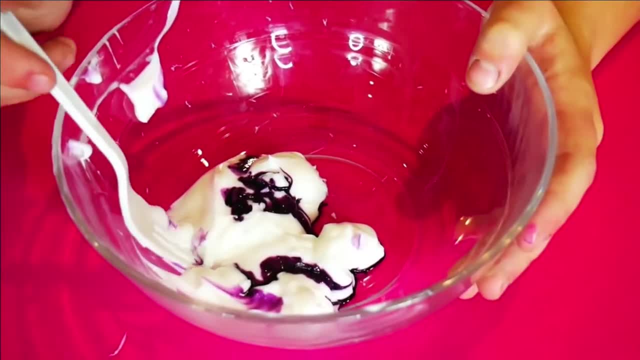 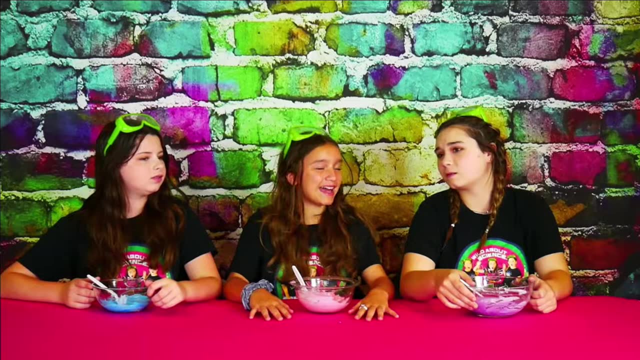 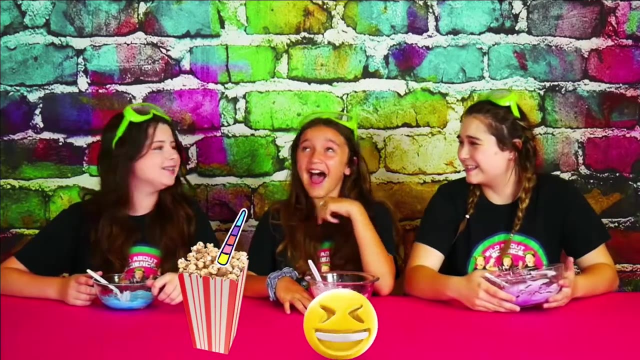 It's like the unicorn mane. Now for my unicorn purple. That is a great purple. Hey girls, what do unicorns call their dads? What Popcorns, Popcorns. I don't know how I came up with this. 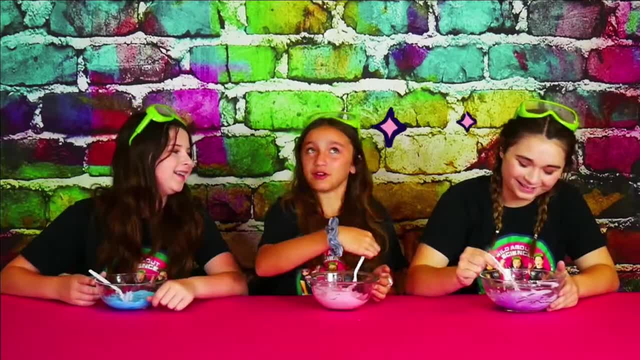 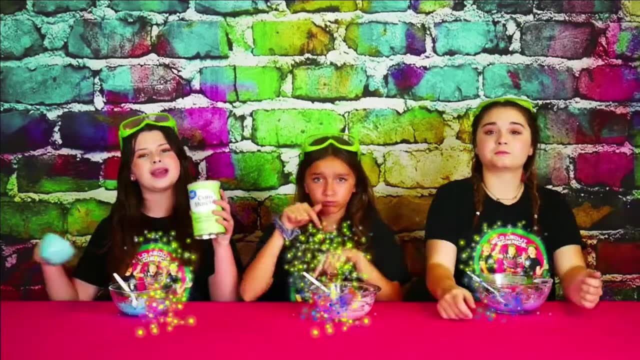 I'm just so good at this. I'm a clever little unicorn. I'm a clever corn. Now that our unicorn cone is ready, it's time to add one cup of cornstarch and mix it all together. Oh yeah, maybe it's time to get a unicorn role. 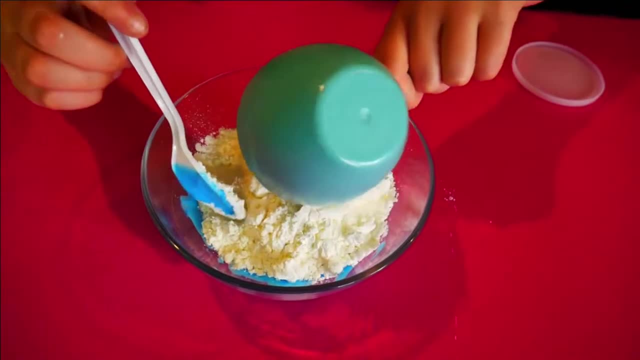 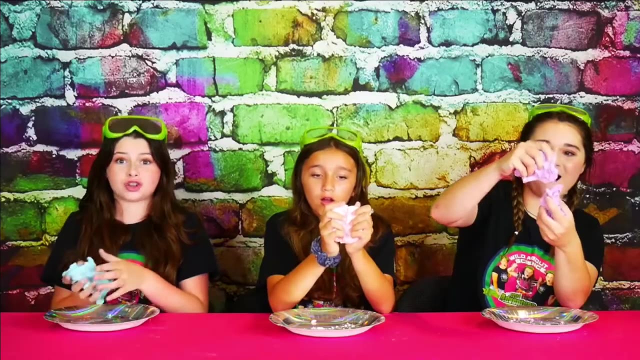 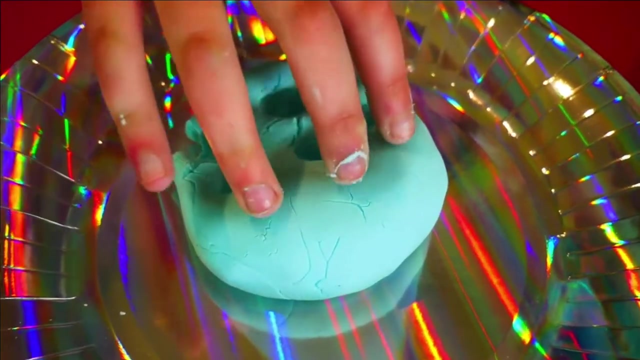 Here's our cornstarch: Whoa, And now we're going to mix it all together. Whoa, This is so soft On the inside it looks like a cloud. Whoa, look how soft this is. Whoa, it looks just like a cloud. 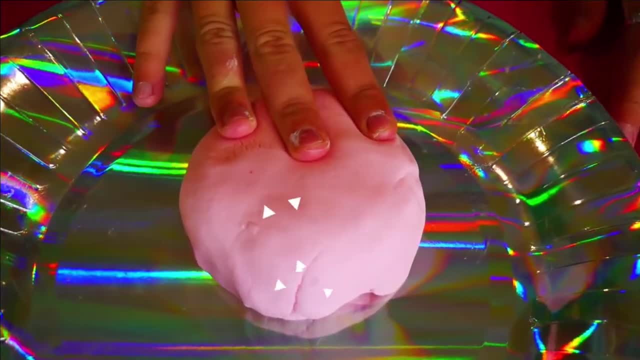 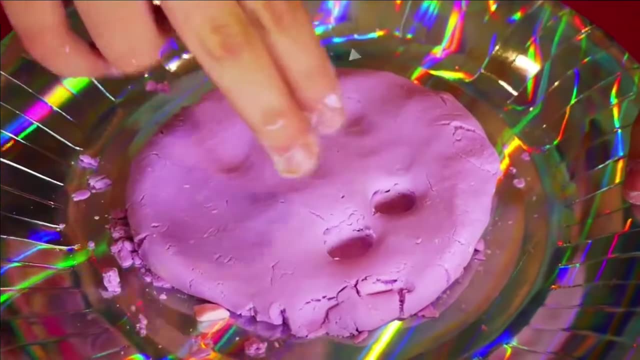 It looks like clay It is. Oh, look how soft mine is. Whoa, You can see your fingerprint. Oh, that is so cool. Definitely can play with this stuff for hours. Ooh, Look how cute this looks when you stack it all together. 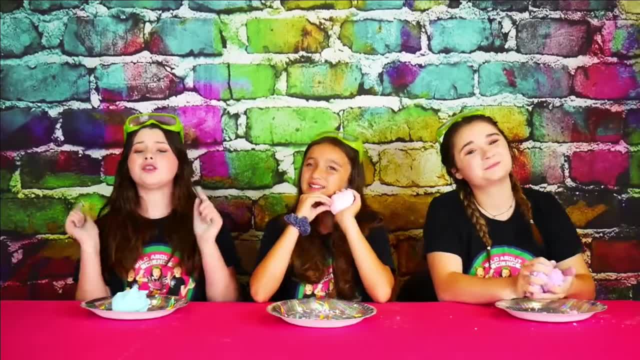 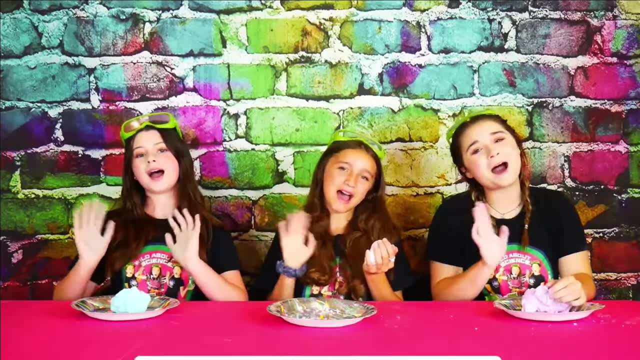 It's so pretty, It looks so cute, you just want to eat it. Overall, we give this unicorn cloud dough a big thumbs up. Okay, bye-bye. Thank you for watching our show. Subscribe to our channel. Bye-bye. 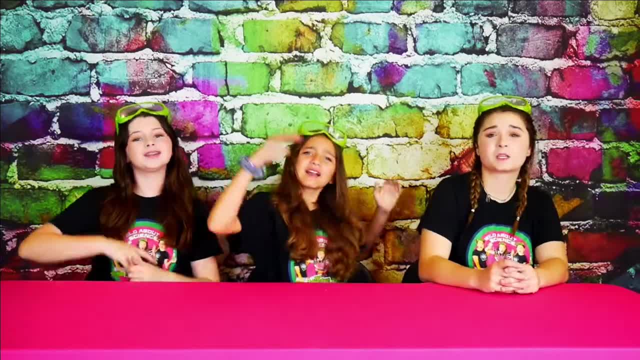 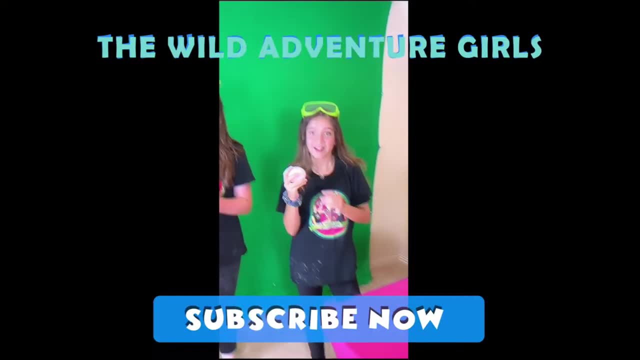 Hi, we're the Live Inch Girls. We're the Live Inch Girls. I'm Alton Torewater. Live Inch Girls Explored. Okay, Okay, Okay, Okay. Second chance tonight to get the good life right. All I need is no more holding on. 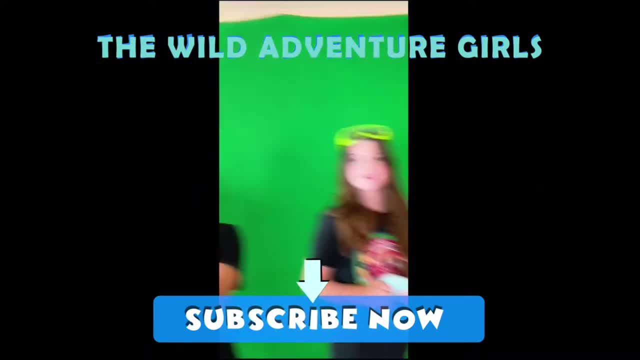